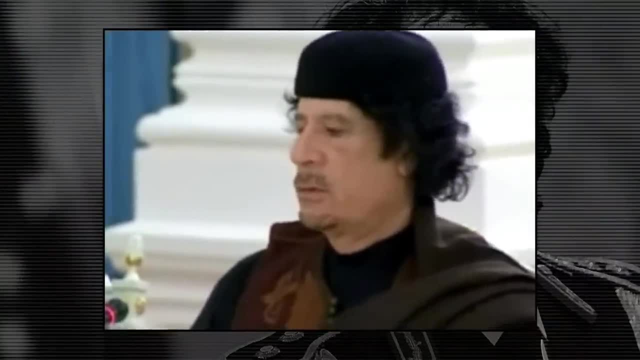 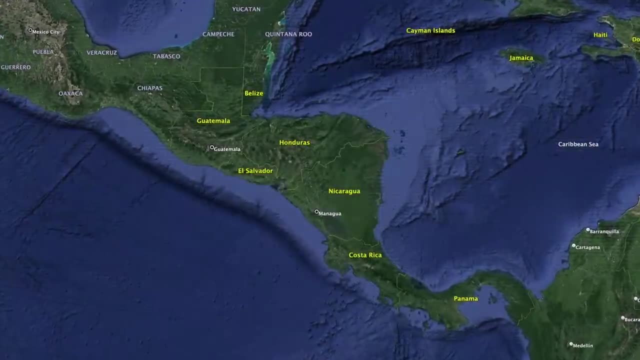 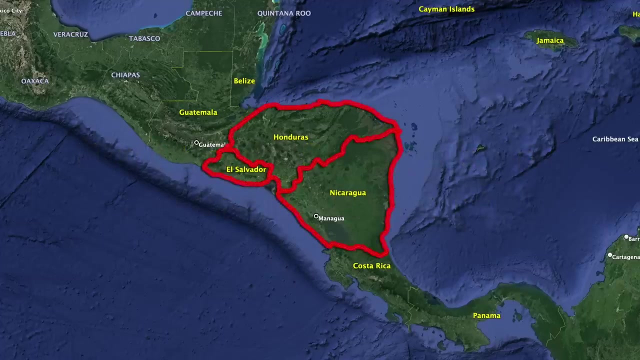 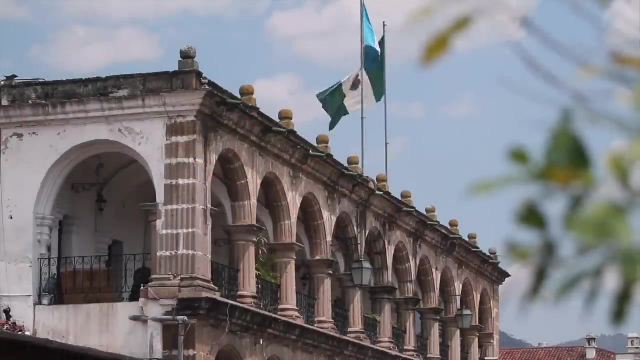 a non-government country. The United Nations Charter states that if a government tries to protect institutions that no longer have property, visitations or houses, bueno, it's considered an upholding of aそれでは Tsantamoura state. It was renamed the United States of Central America when its constitution went into effect. 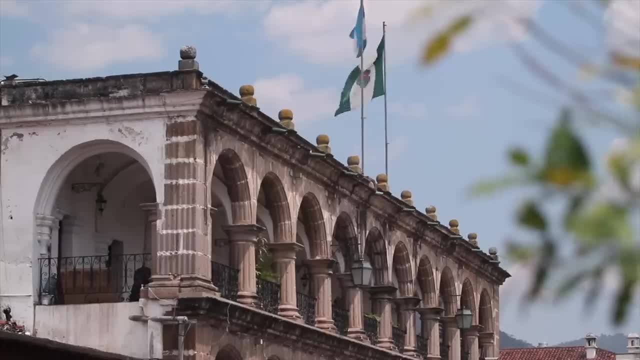 on 1 November, Norman C Hamilton, When the government of the United States of Central America was running the state to the consent of the zasadist Republican National Party, 1898,. but the country was dissolved just 28 days later when El Salvador experienced a military. 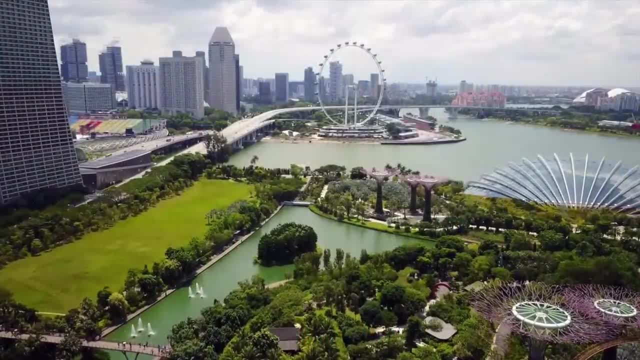 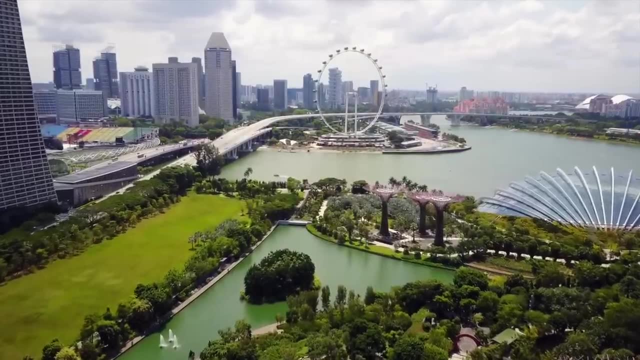 coup by this guy. Singapore's constitution requires the president to have at least three years of experience in a high-ranking government job, or three years as chairman of the board or CEO of a company worth at least half a billion dollars or an important government company. 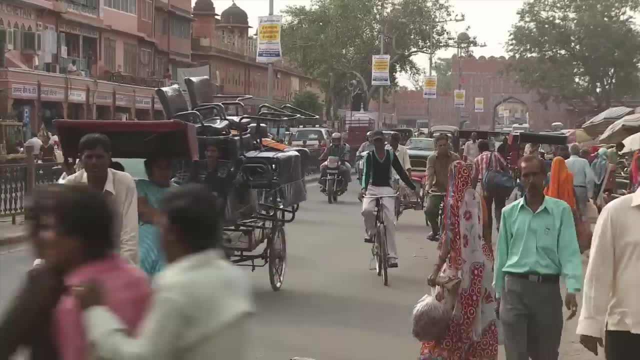 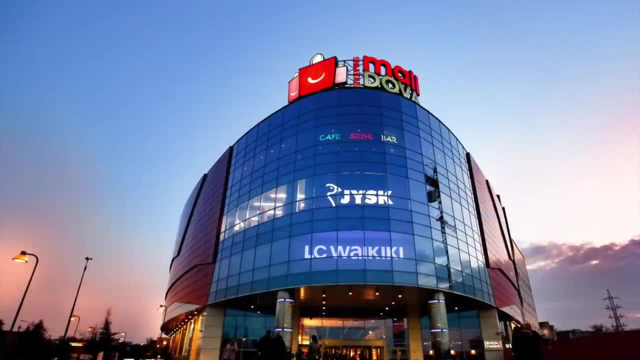 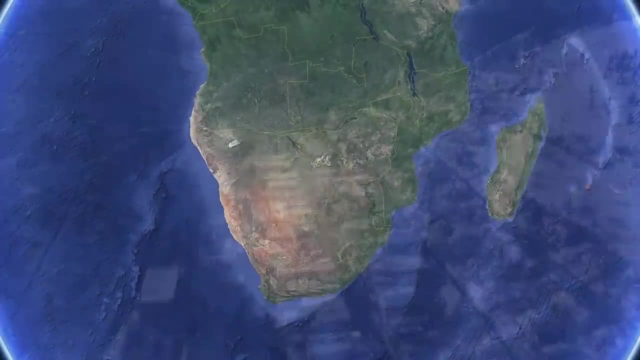 India has the longest written national constitution in the world, at about 145,000 words. Moldova has a mall called Moldova. There is a city park in Park City, Utah, called the Park City City Park. In 2021, Botswana had the highest GDP growth rate of any sub-Saharan. 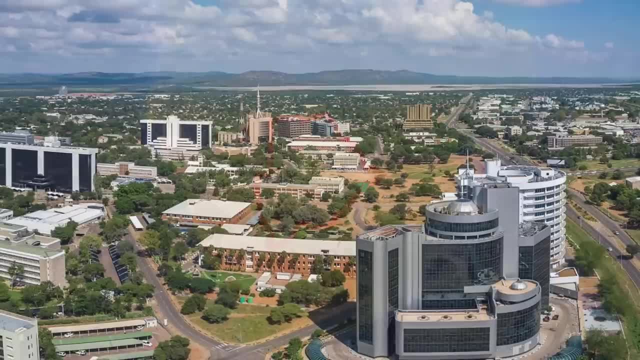 country at 12.93%, but their growth slowed to an expected 4% this year. This is partially due to global warming. India has the longest written national constitution in the world, at about 12.93%, but their growth slowed to an expected 4% this year. This is partially due to global 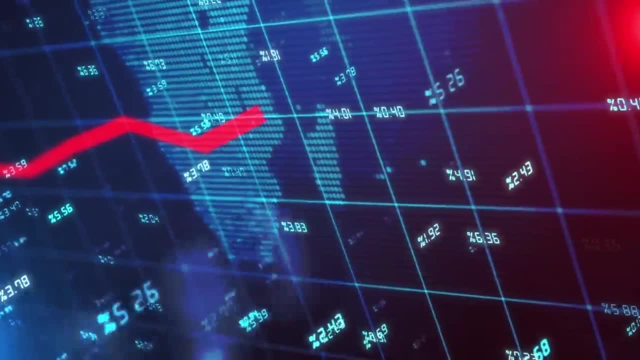 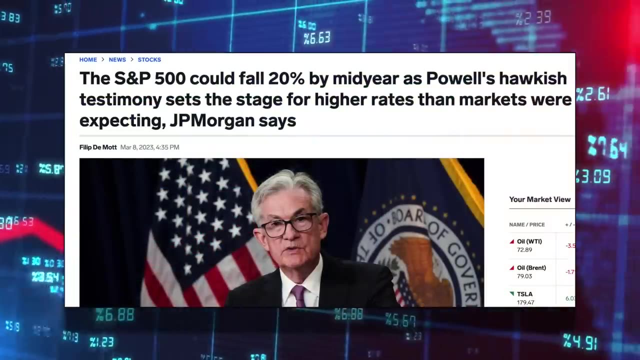 inflation And, the worst part, How inflation has affected the average person, including their investments, which are plummeting, like the stock market, which is either going to flatline or lose 20% depending on which major bank you ask. Historic times, but Masterworks has been helping. 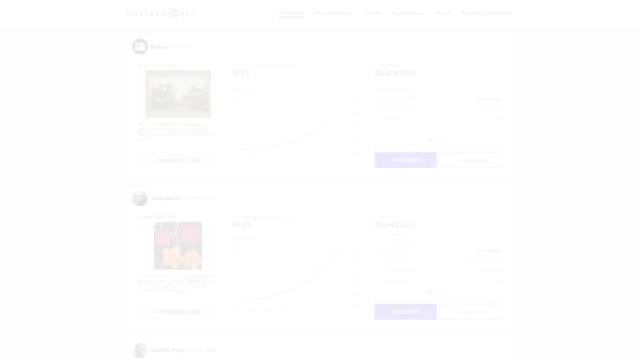 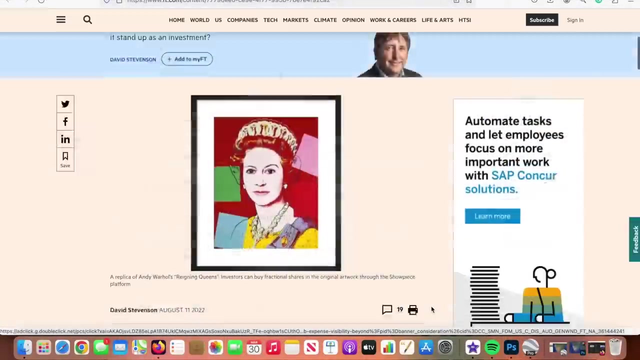 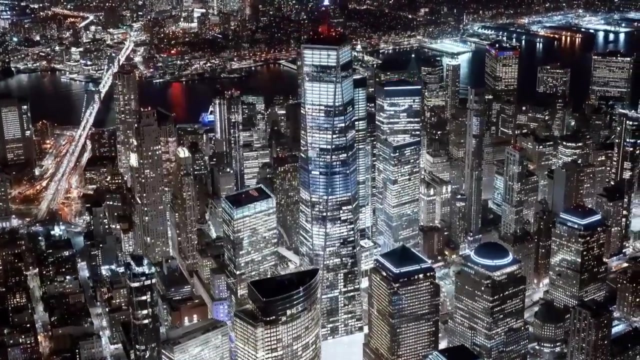 over 650,000 people adapt through it, all paying out tens of millions in returns last year alone. No wonder they've been featured in financial publications like Business Insider and Financial Times and were recently awarded one of LinkedIn's top 50 startups Because, from Masterworks' office in downtown Manhattan, their team 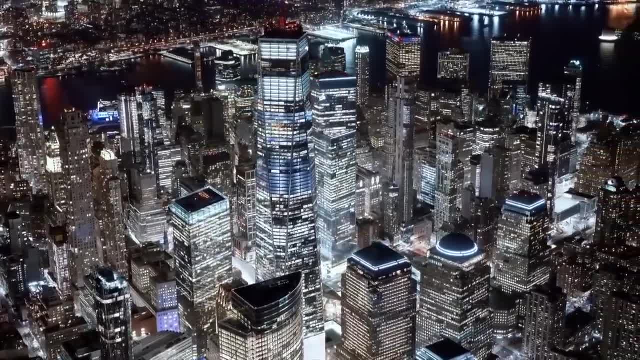 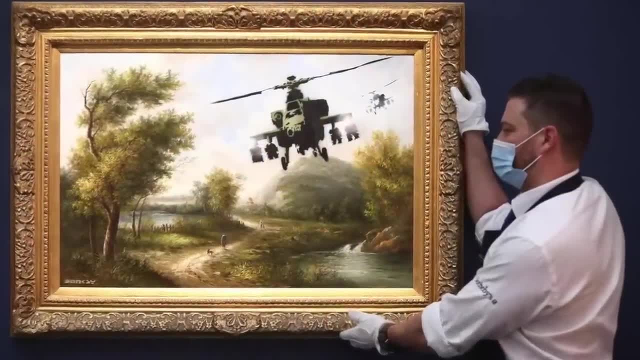 is revolutionizing art investing Now. I was skeptical when they first approached me earlier this year, but Masterworks doesn't do NFTs or crypto. You're investing in real physical paintings from legends like Picasso and Banksy, And they're qualified with the SCC. 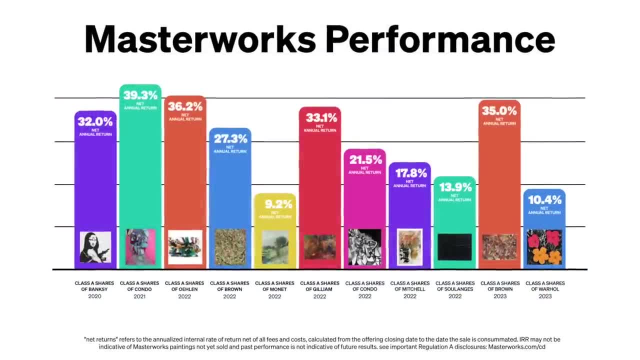 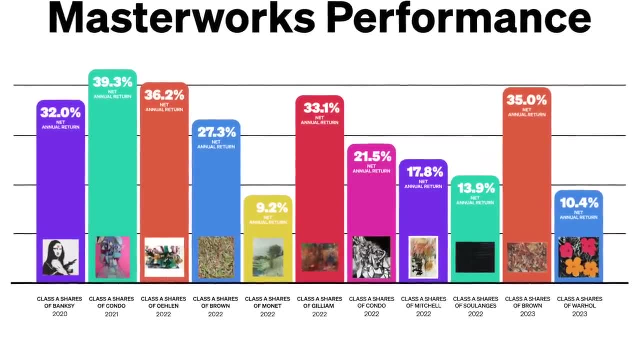 which I've linked in the description. In fact, some of you may have seen a return from Masterworks. They've sold eight paintings since we partnered in July, for a total of 11 sales to date, And right now my viewers can claim a complimentary Masterworks account. 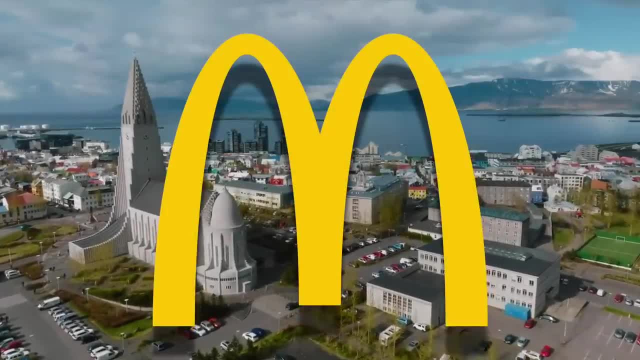 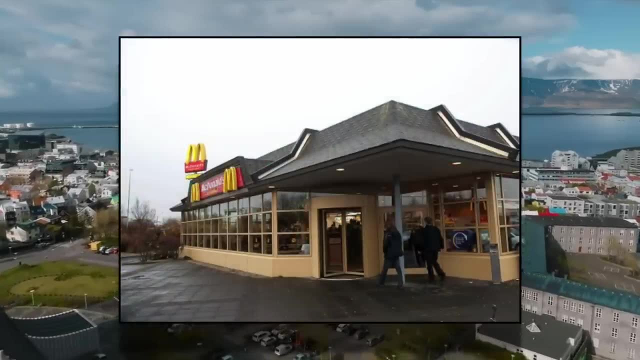 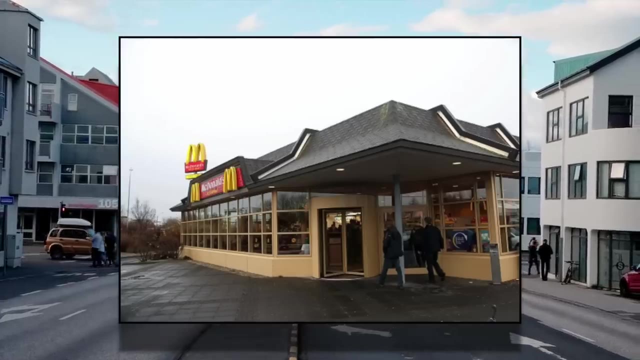 just by signing up with my link below. There are no McDonald's in Iceland, But that wasn't always the case. The first McDonald's in Iceland was opened in 1993.. But 16 years later, when the Great Recession hit, import prices to Iceland skyrocketed And so the company closed. 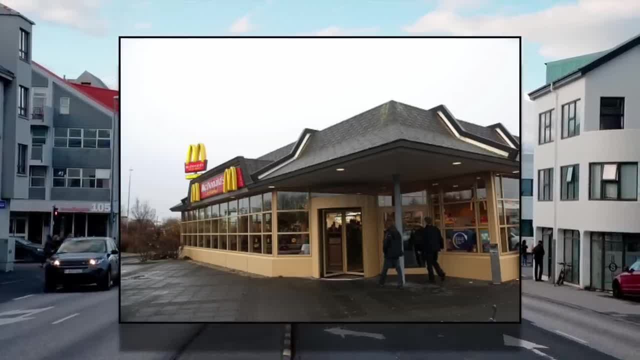 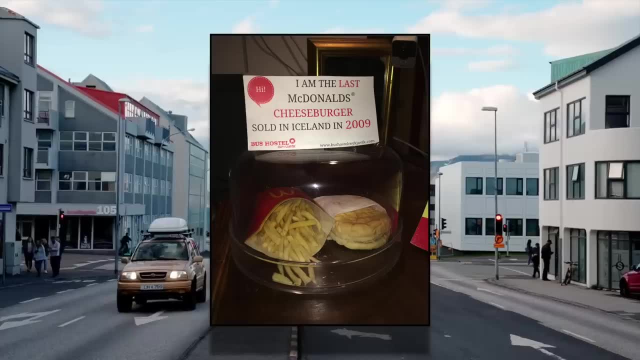 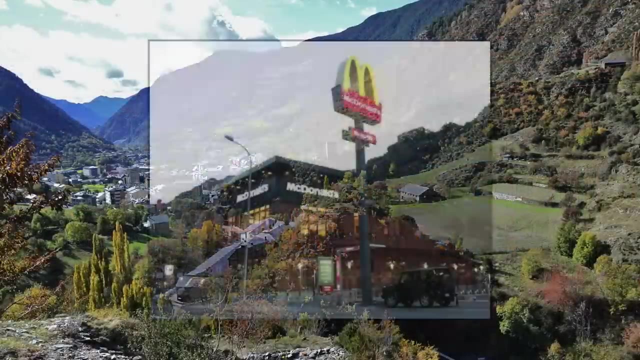 all its restaurants in the country. Iceland hasn't had a McDonald's since 2009.. The man who bought an Iceland McDonald's never ate the burger. He wanted to see if it would ever decompose. That burger is now housed at the Snartra House, a hostel in southern Iceland. 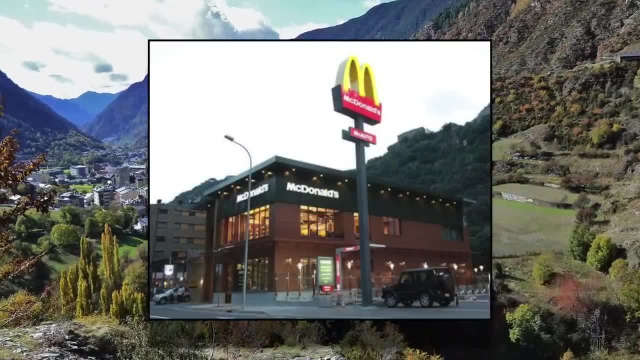 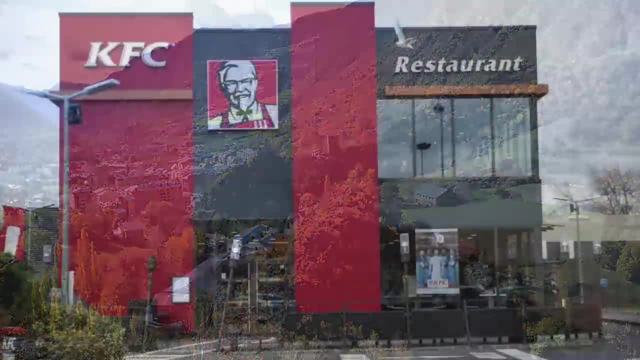 Andorra has five McDonald's And, because of its low population of around 80,000 people, this means Andorra has more McDonald's per capita than any other country. In 2009,, KFC sent a letter to the United Nations asking for membership under the name Grilled Nation. 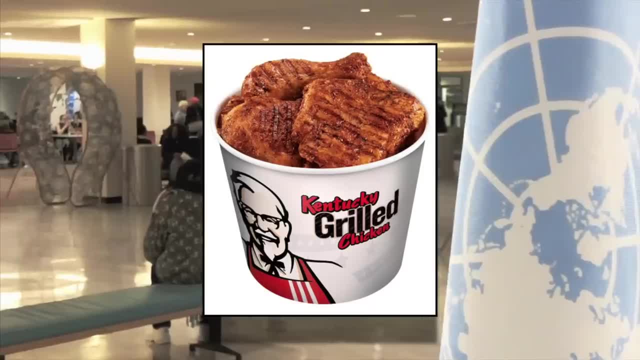 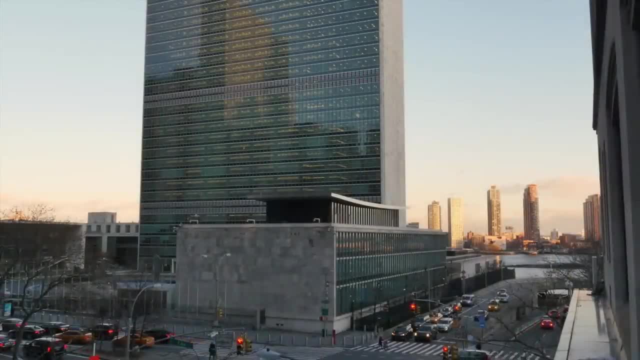 which represented 60 million people who would like to be part of the Grilled Nation, And they did. As what would have been the 193rd member country. the nation would have given free samples of grilled chicken across the street from the UN headquarters in order to promote. 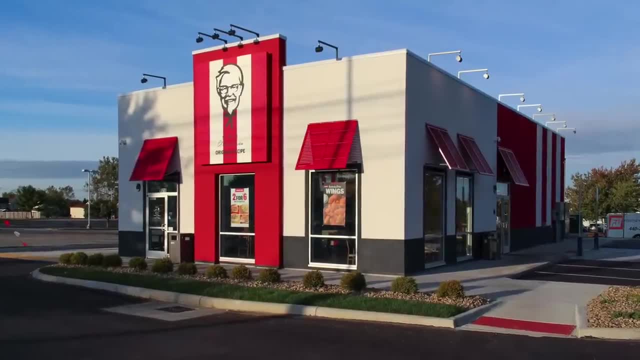 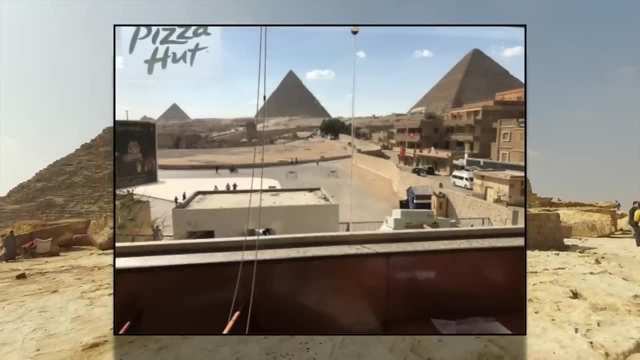 Monday's in-store free piece of grilled chicken event, The Grilled Nation was not admitted. There is a KFC as well as a Pizza Hut, with a view of the Pyramids of Giza. The tiny island nation of Tuvalu consists of nine islands, But Tuvalu means 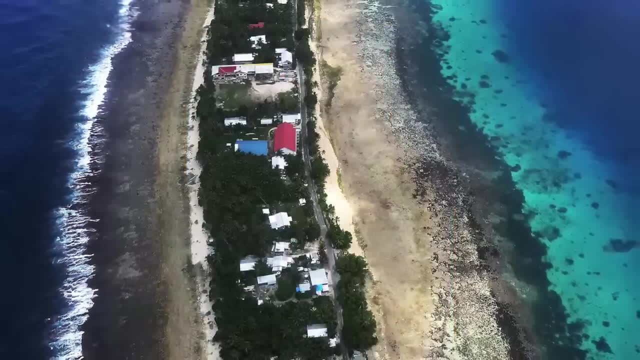 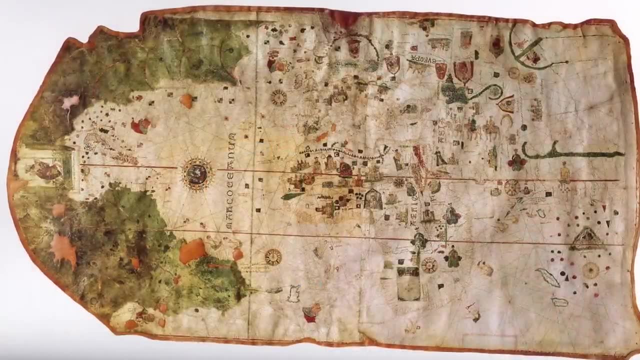 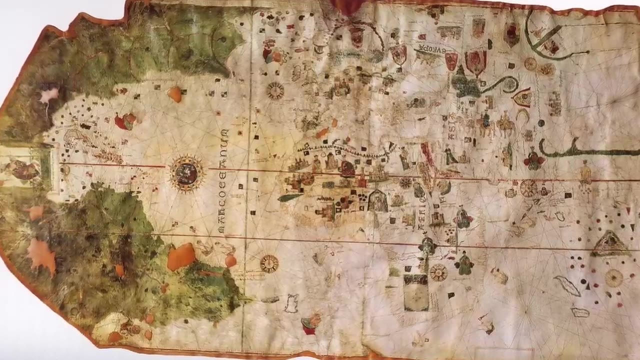 standing together in Tuvaluan. This is because only eight of the islands were populated. pre-European contact: This map was likely created in the year 1500, and it's the earliest known representation of the New World and the first depiction of the equator on a nautical chart. The map. 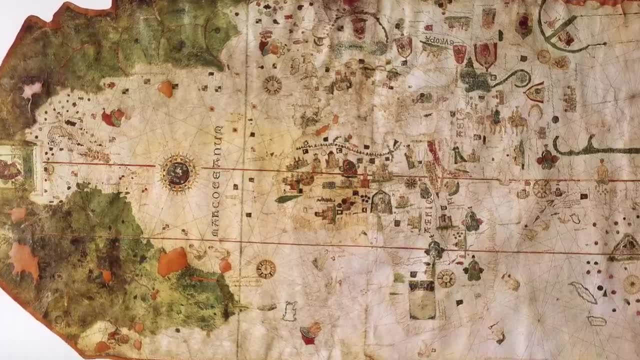 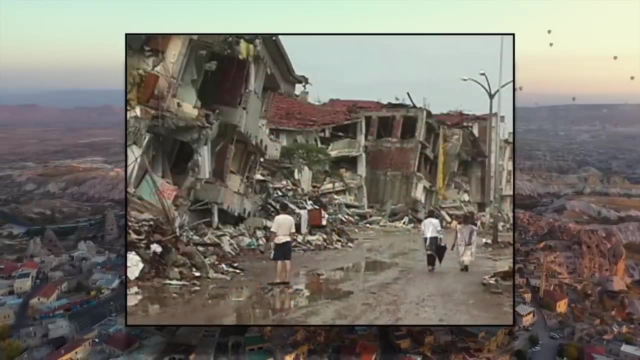 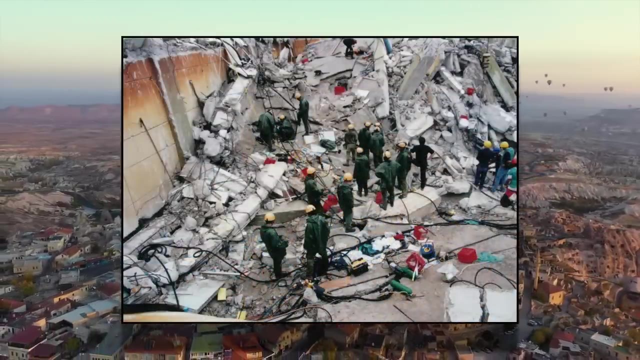 is attributed to the Castilian navigator and cartographer, Juan de la Casa. Greece and Turkey have what's being called earthquake diplomacy, After both countries were hit with successive earthquakes. in the summer of 1999, the countries agreed to help each other in the case of an earthquake, no matter how bad their relations are. 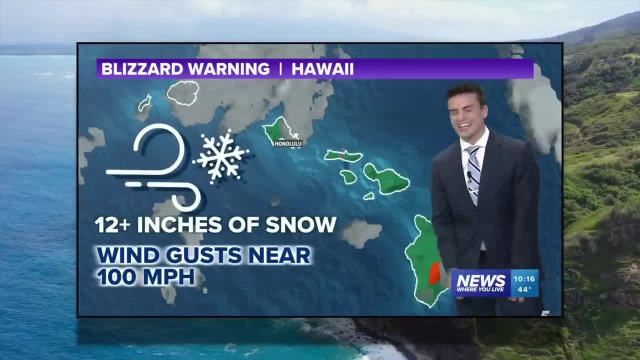 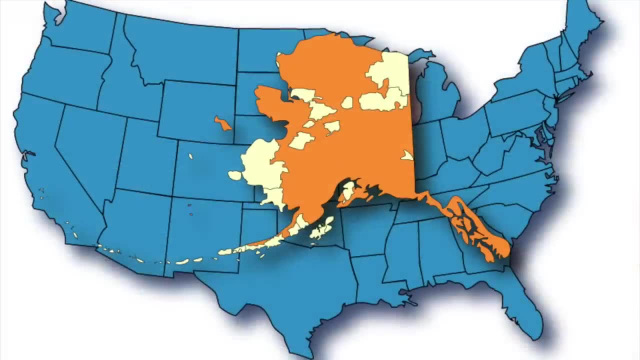 Hawaii is in the tropics, where the length of day and temperature is generally warm throughout the year, But at its highest elevations an occasional blizzard can occur. The United States largest state, of Alaska, is bigger than the next three largest states combined- Texas. 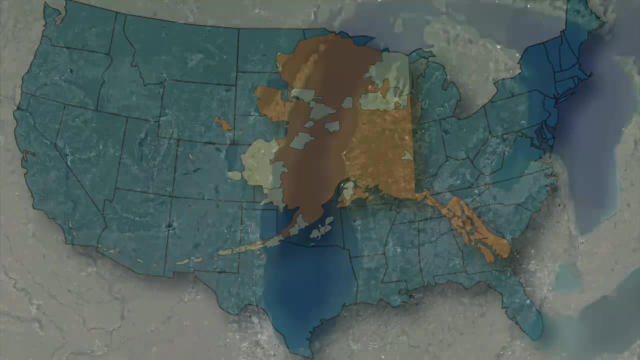 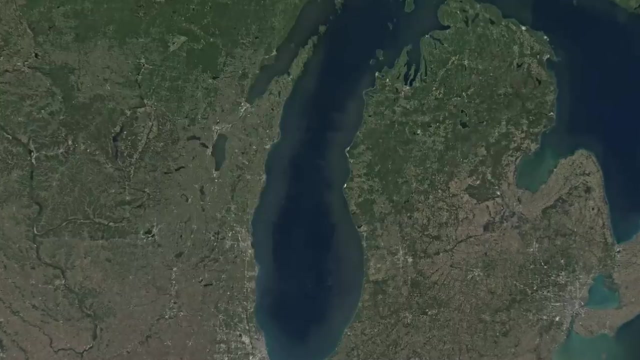 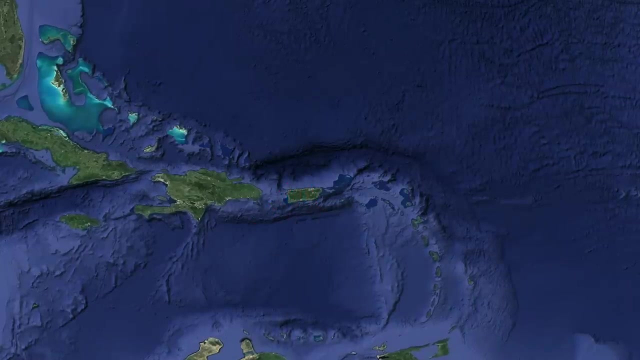 California and Montana. An estimated 300 trillion invasive mussels blanket Lake Michigan, but it's down from its peak of 480 trillion nearly 20 years ago. The Puerto Rico Trench, located on the periphery of the Caribbean Sea, is the deepest in the Atlantic. The trench is 800 kilometers long and has a maximum depth. 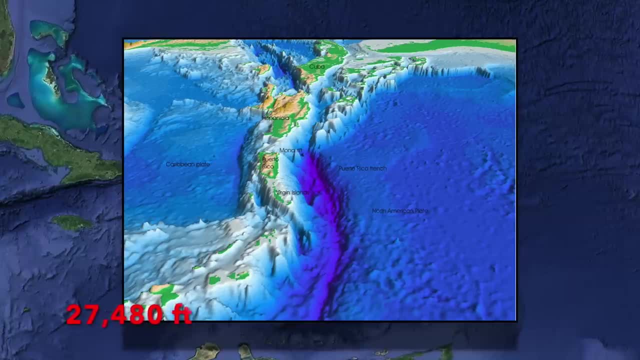 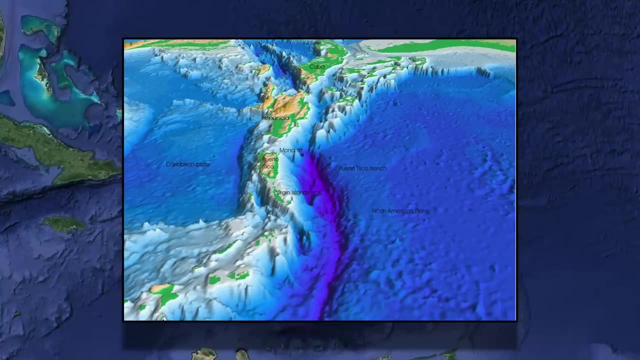 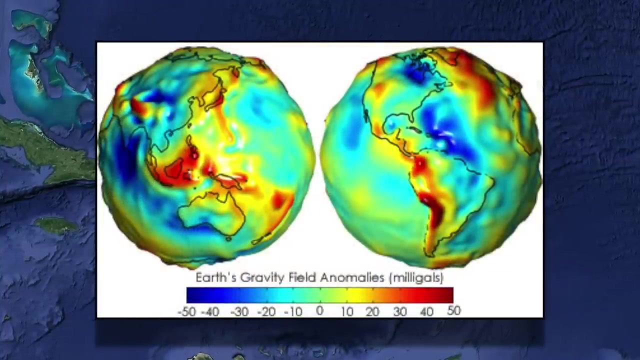 of 8,376 meters. This point is, of course, the single deepest point in the Atlantic Ocean. It's commonly referred to as the Milwaukee Deep. According to NASA, beneath the Puerto Rico Trench is a mass so dense that it's caused the location. 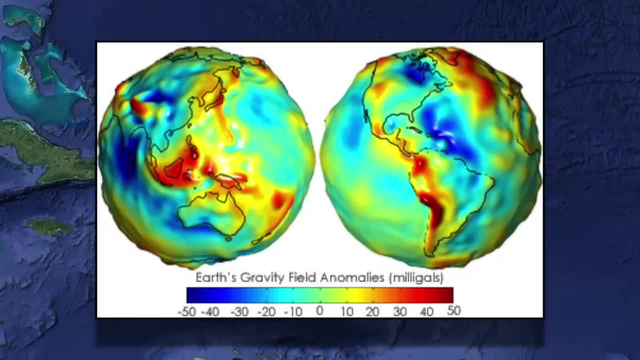 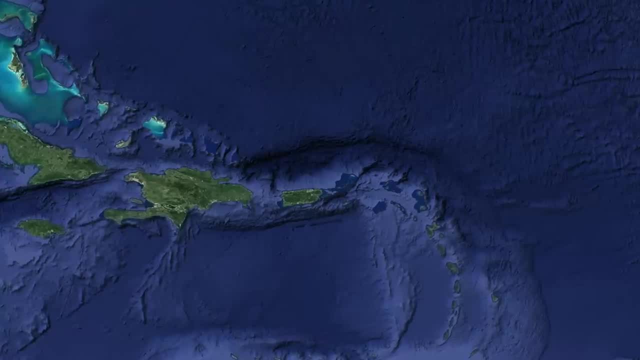 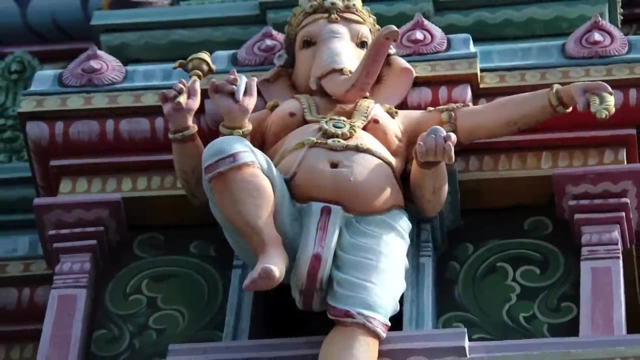 to be the biggest gravity anomaly on Earth, meaning that, because of its location, there should be less gravity, but something is creating a greater pull. This has also been known to have a negative effect on the accuracy of navigational instruments. Forty-eight point five percent of 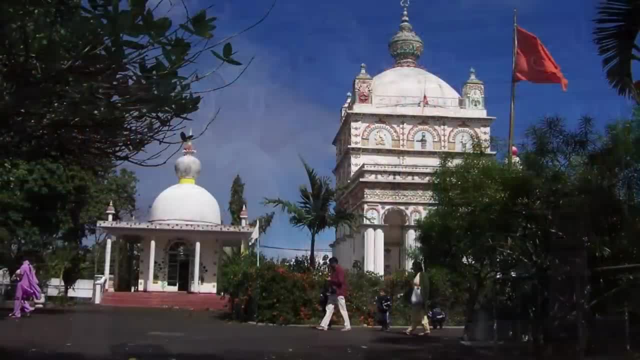 people on the island nation of Mauritius are more likely to be affected by an earthquake than by a tsunami. The top five places this can happen in Mauritius are Hindu, making it the only country in Africa where Hinduism is the most followed religion. 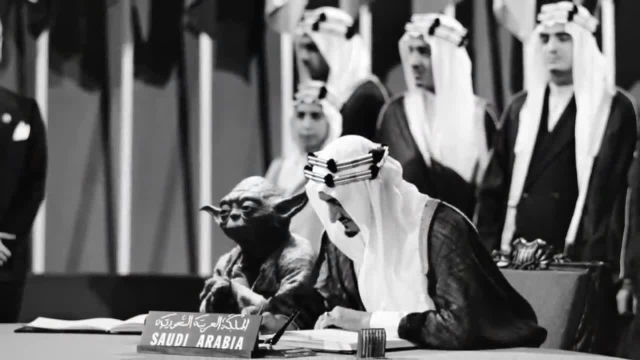 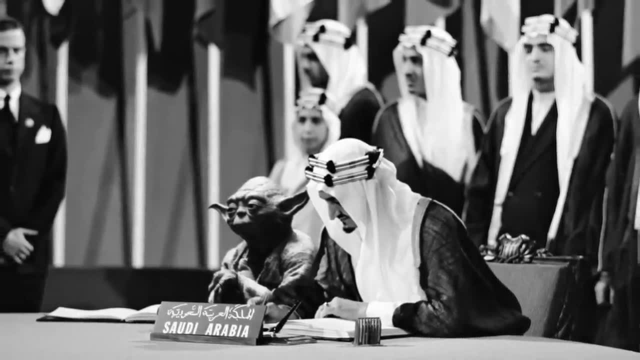 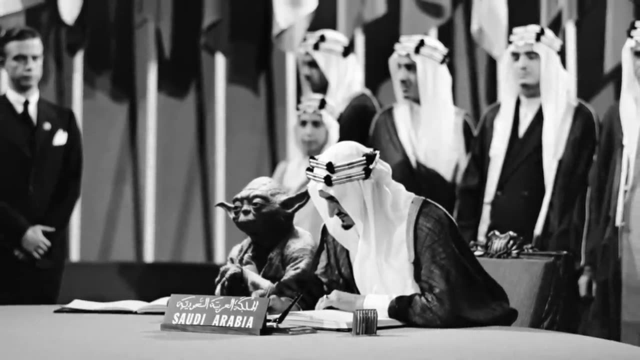 In 2017, Saudi Arabia accidentally published a school textbook with the Star Wars character Yoda, seen photoshopped next to the late King Faisal as he signed the UN charter in 1945. Saudi Arabia's Education Minister publicly apologized for the mistake. The Appalachian Mountains on the eastern 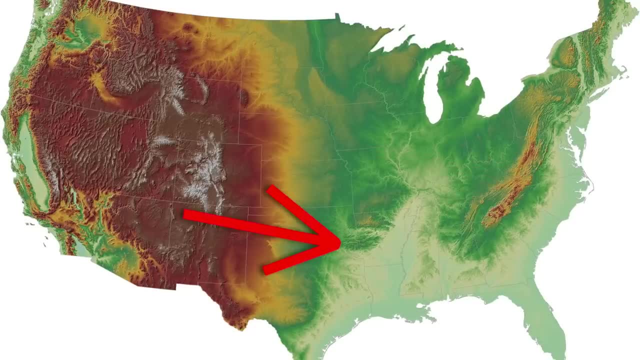 side of the United States are the most popular tourist attractions in the world. The islands in the North and the South are the most popular tourist attractions in the world. The United States has the States the Ashita Mountains in Arkansas and Oklahoma and the Little Atlas Mountains of. 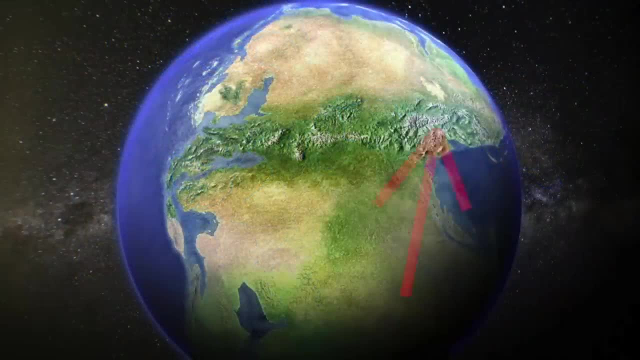 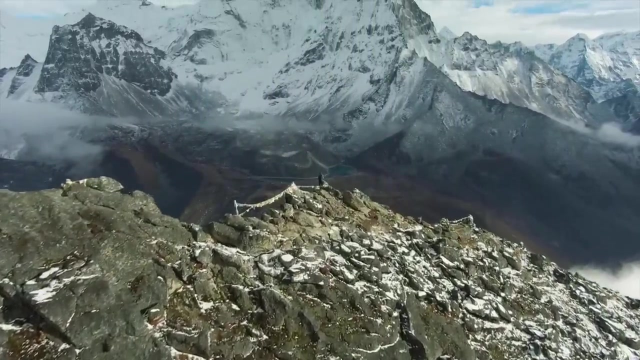 Morocco all used to be part of the same mountain range, the central Pangean Mountains on the supercontinent of Pangea. This mountain range began forming around 340 million years ago and had reached its greatest elevation at around 295 million years ago. At its greatest elevation, 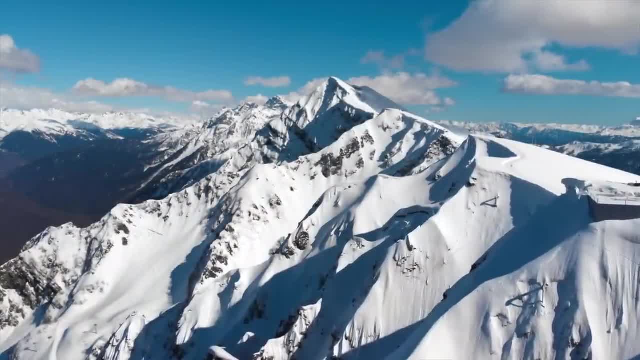 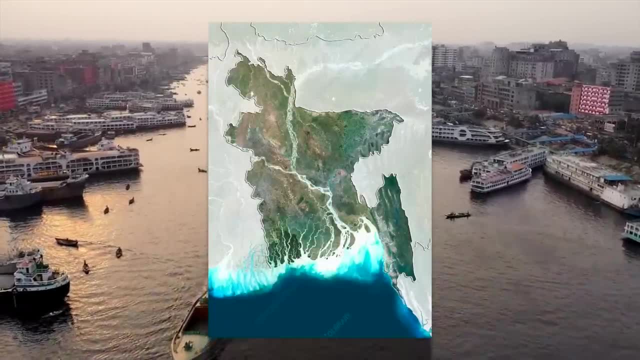 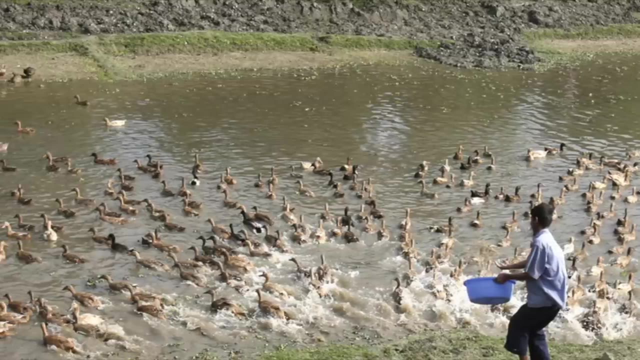 it was around the same height as today's Himalayas. Bangladesh is a flood-prone country due to being situated on the Ganges Delta and the many distributaries flowing into the Bay of Bengal. Many chicken farmers have had enough and are changing to raising ducks because if their 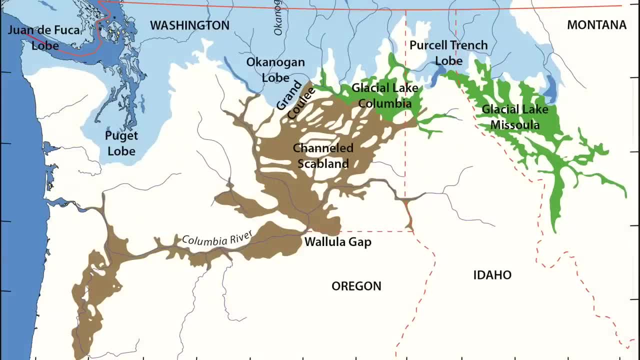 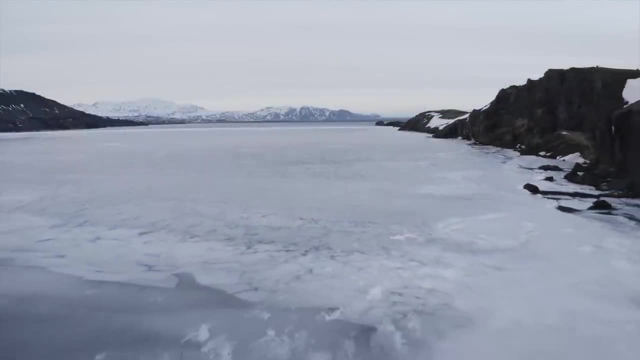 farms flood, the ducks will float. Between 15 and 13,000 years ago, there was a lake that existed periodically in what is today western Montana called Lake Missoula. The lake measured around 3,000 square miles and contained about 500 cubic miles of water. 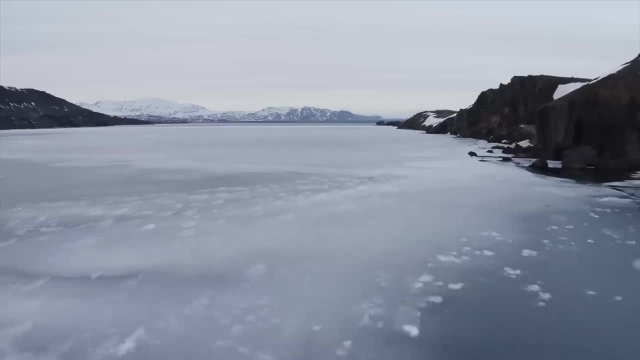 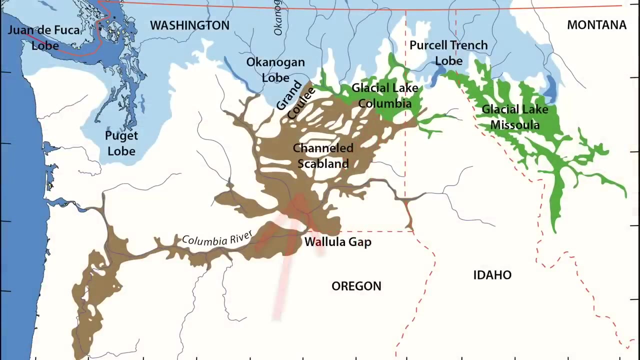 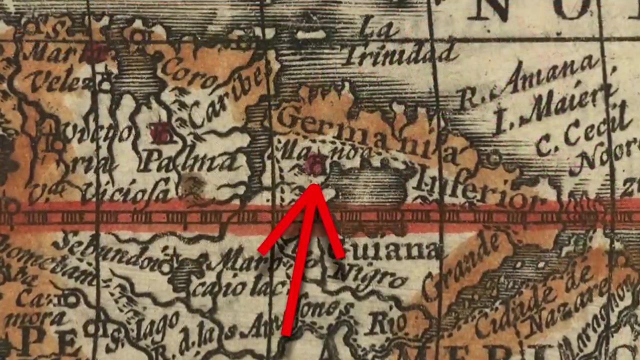 The lake was the result of an ice dam. The ice dam would occasionally break, sending water through the glacial Lake Columbia and causing catastrophic floods in what is today Washington, Idaho and Oregon. It's believed that this occurred around 40 times. El Dorado is named on many 16th. 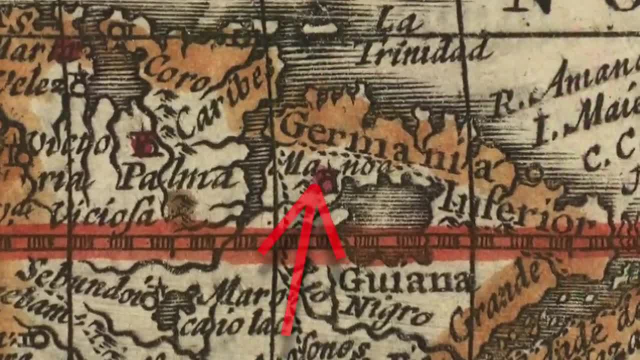 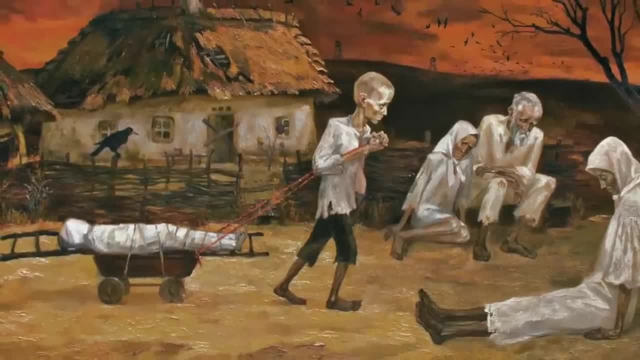 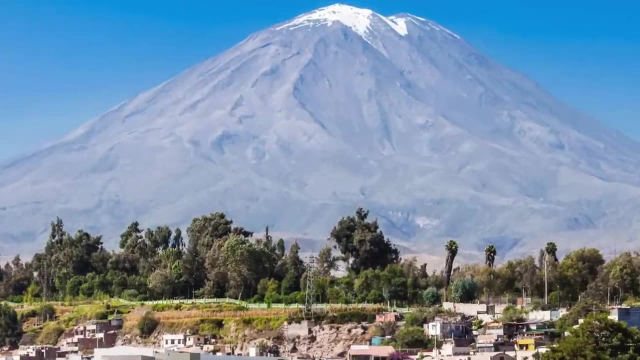 and 17th century maps, but often as the name Monaco. 2 million people, which was nearly one-third of the Russian population, died of starvation from 1601 to 1603 due to a volcanic eruption. The volcanic ash obscured the sun, destroying the crops. That volcano was located in Peru. 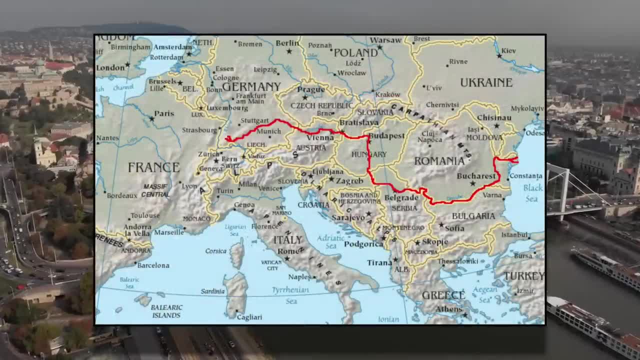 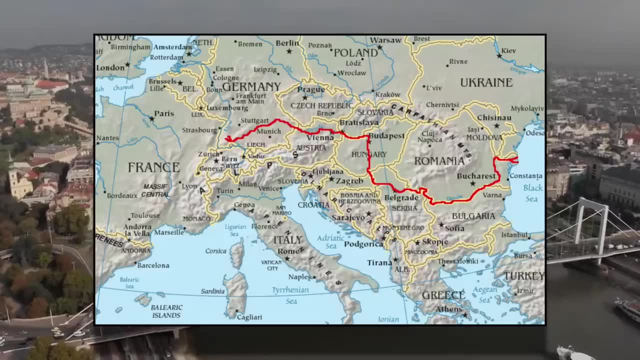 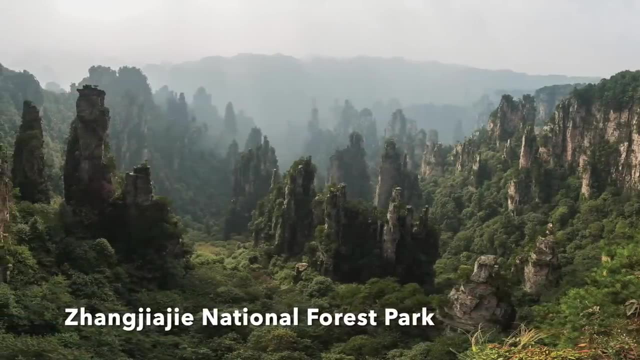 The Danube passes through the most countries in the world, crossing 10 countries: Germany, Austria, Slovakia, Hungary, Croatia, Serbia, Romania, Bulgaria, Moldova and Ukraine. China created its first national park in 1982.. The park is best known for its 3,000 vertical. 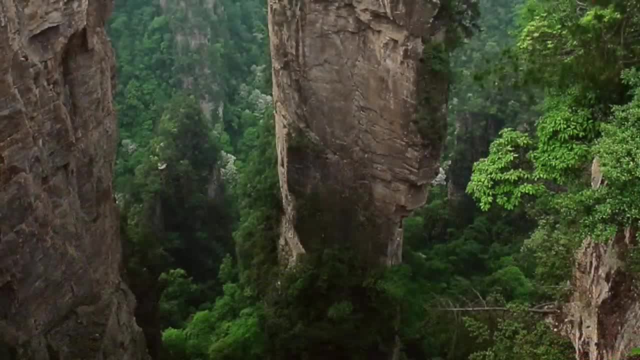 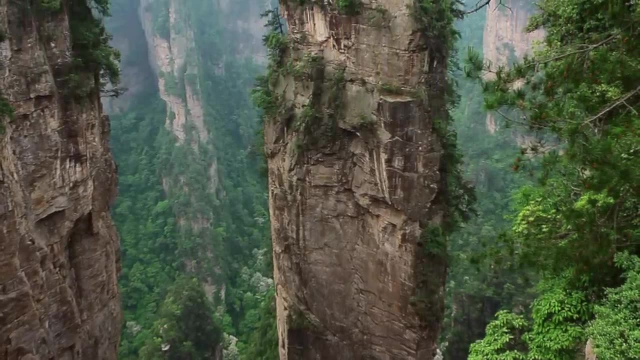 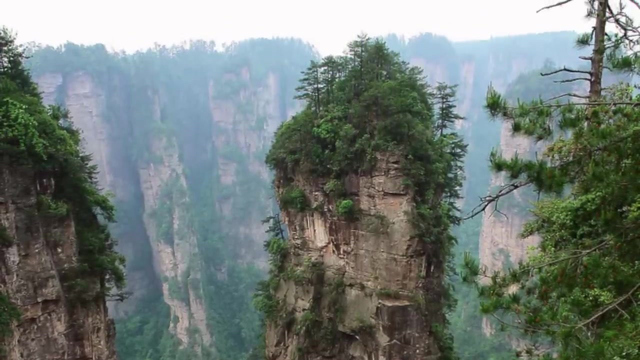 pillars standing hundreds of feet tall. One of these pillars, which stretches 3,544 feet into the air, was named the Southern Sky Column, But in 2010, the name was changed to Avatar Hallelujah Mountain, after the highest-grossing film of all time, Avatar, used the pillar.